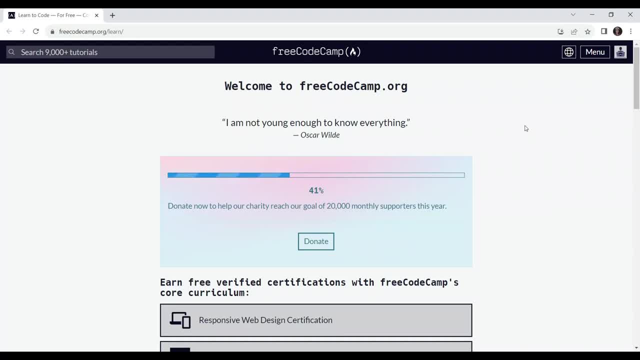 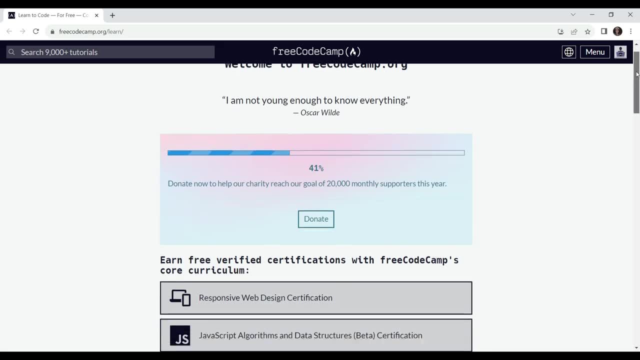 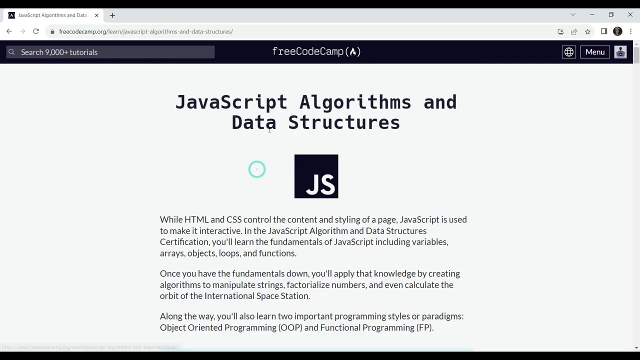 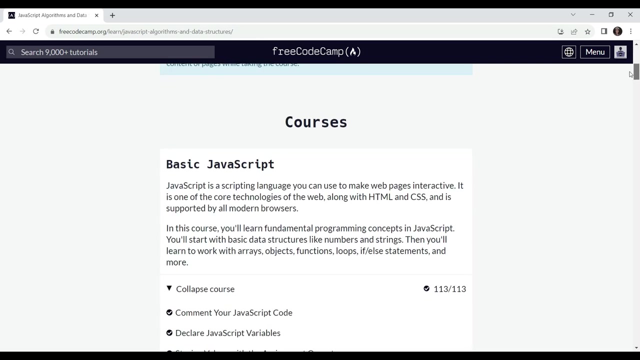 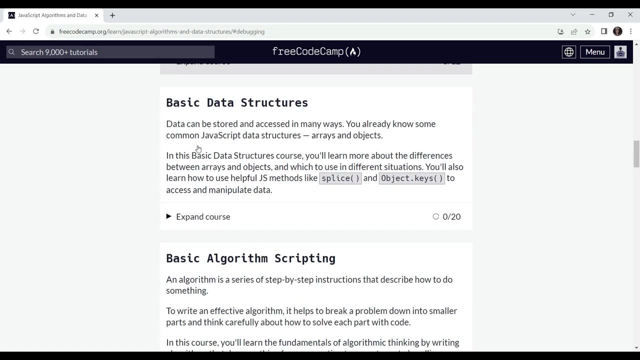 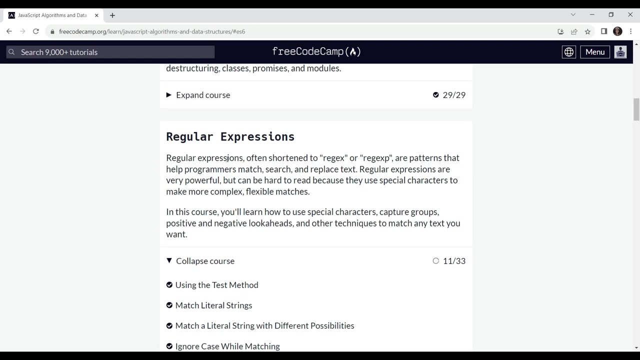 Today on FreeCodeCamporg, we'll be exploring the JavaScript algorithms and data structures course in the Legacy Curriculum section. More specifically, we'll be taking a look at the Regular Expressions module. Today we'll be doing steps 1-11 in this module. 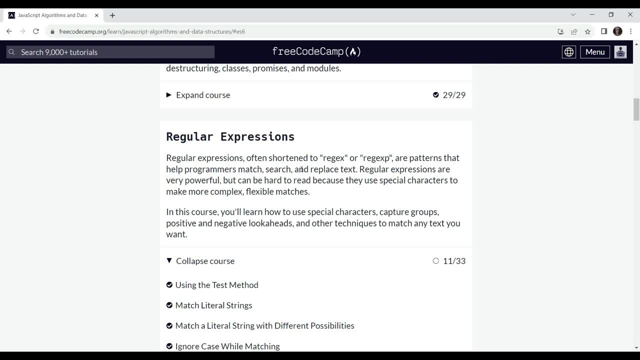 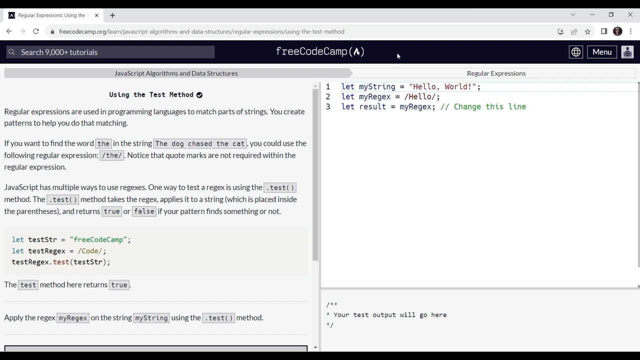 Regular Expressions are also known as Regular Expressions. Regular Expressions are also known as Regular Expressions. Regular Expressions is a viagra. that means the. we want to test. we want to test, we want to use and apply the test, the dot test method, to evaluate whether a particular object 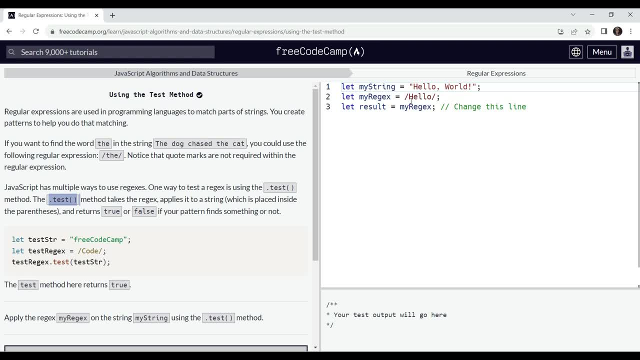 is contained in a string. for example here: object: my string is equal to hello, comma world. and then the next object, my regex, is equal to hello, contained in the single slash syntax. so we're going to let the result be equal to: according to this syntax here given in the example we're 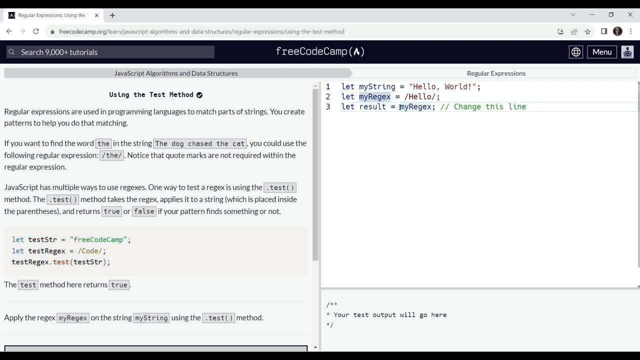 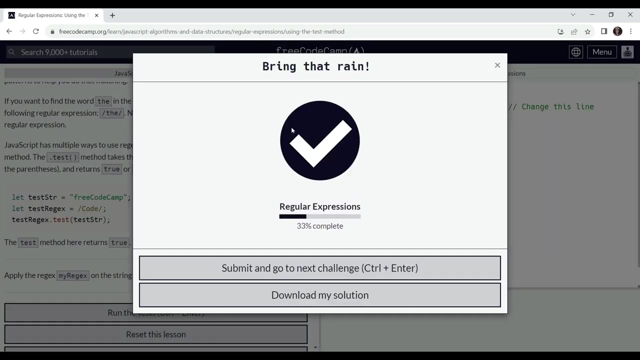 going to let the result be equal to first the my string object, because we're testing to see again if my regex, if hello, is contained inside of the my string object- hello comma world. so we're going to give that a go. we're going to run the test and it worked. match literal strings, so the 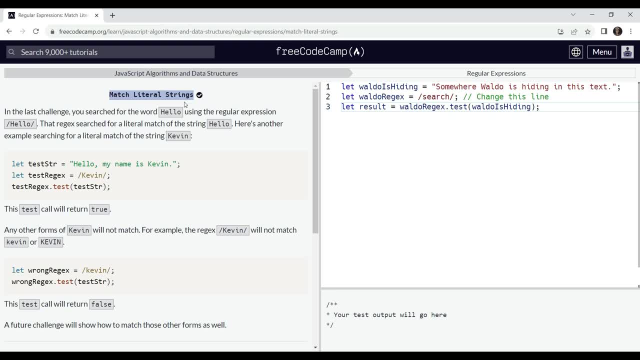 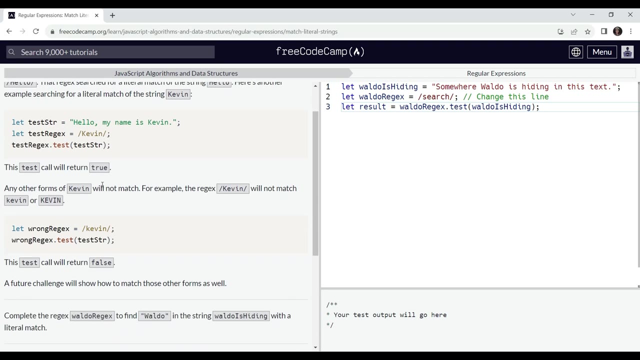 idea with this step is we're going to still implement the dot test method, but this time it's this: met. this step is concerned with the case sensitivity of the search object. okay, so here it's explaining how the test method here will return false, because Kevin is in lowercase, but the 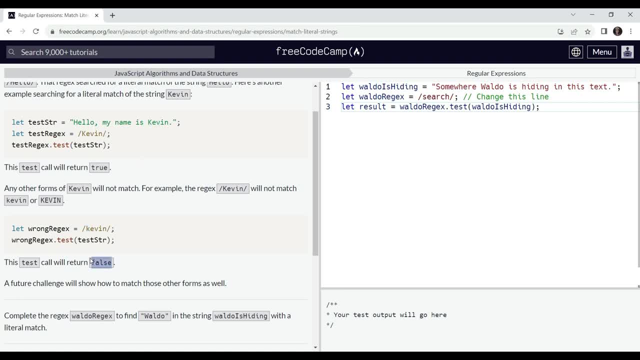 original string has Kevin an uppercase. that's why it returns false. because the case перв an uppercase. that's why returns false. because the case method will return false. because the case suicidator is in lowercase, because when they cases of letters don't match in this test method. 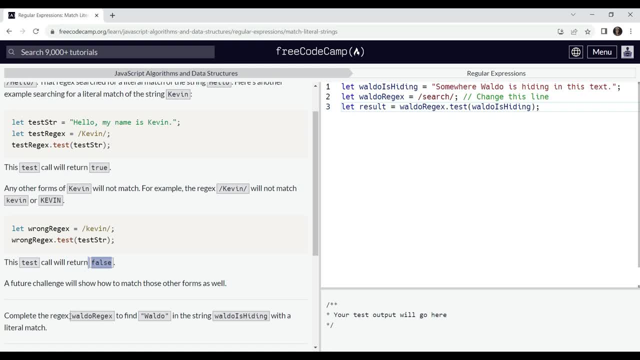 So here it's asking to complete the regex of Waldo regex to find Waldo in the string Waldo's hiding with a literal match. So if we want a literal match, we want this method to return true, of course. So here we want. 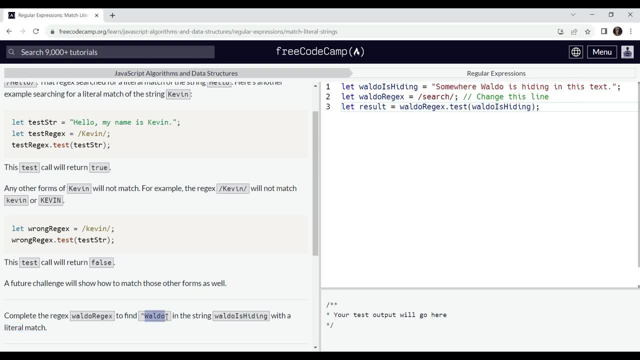 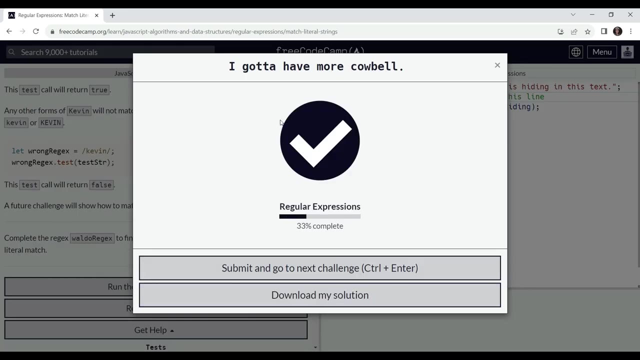 to find Waldo, So we're going to type in Waldo here with the same case. We're going to match cases because we want it to return true, So let's give that a go. And it worked On to the next step. 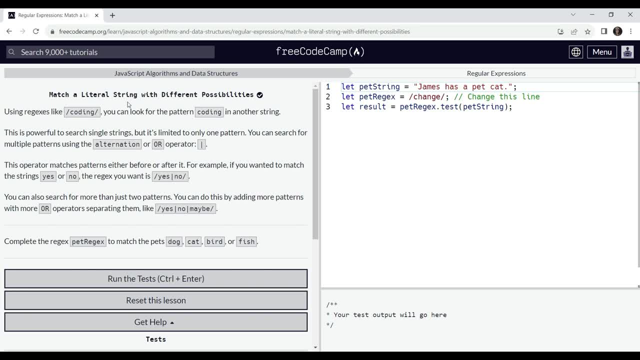 Now this one is asking for the same method of matching a literal string, but now with different possibilities, Meaning with different operators being used. A, yes, no, an or operator are both examples. So here we want to match, we want to use this test function to match. 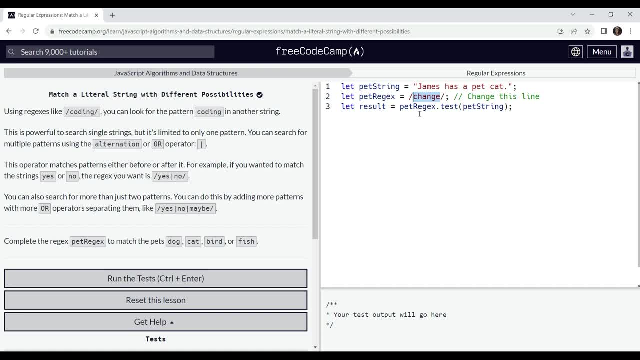 dog, cat, bird or fish. So we'll just match the syntax here given with the or operators, because it says or right here in the prompt. So any of these strings will be considered a match. So we'll write: dog, vertical bar, cat, vertical bar, bird, vertical bar fish. 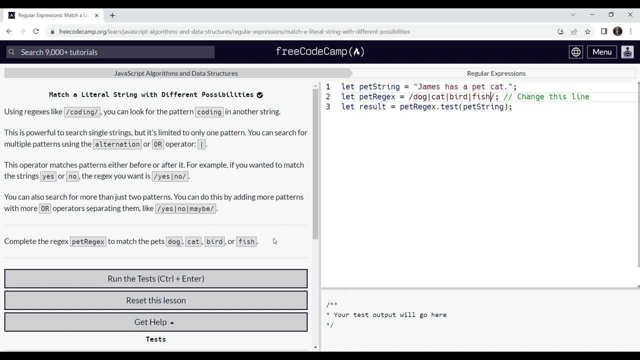 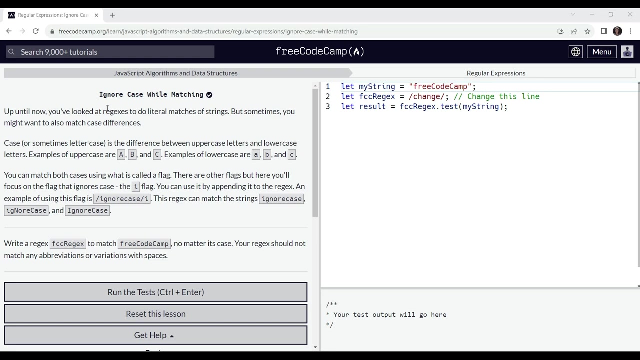 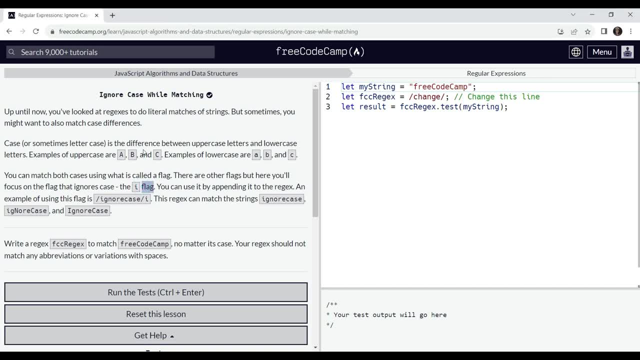 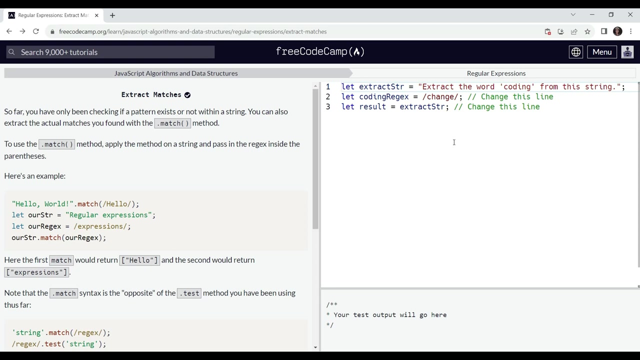 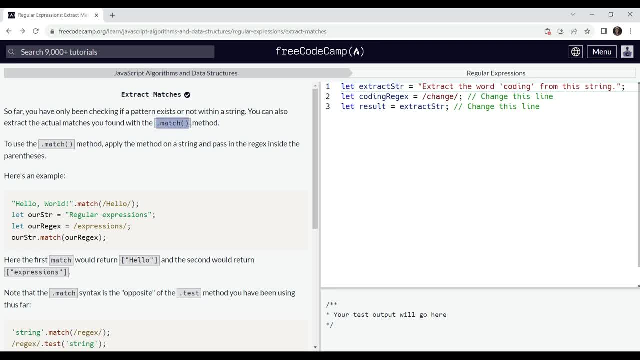 step. this is going to utilize the dot match method, which is actually a little bit different than the dot test method in javascript. so in the dot match method the method is actually applied on a string and inside of it is the actual string or the regex inside the parentheses. 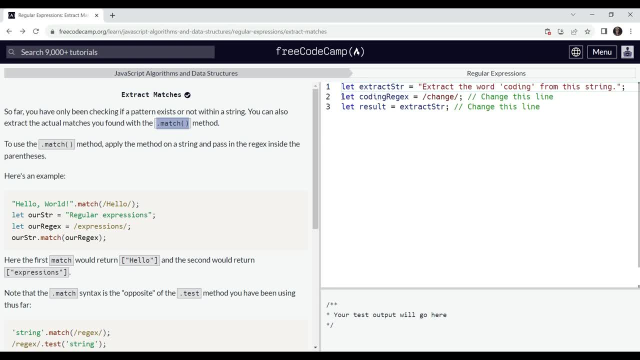 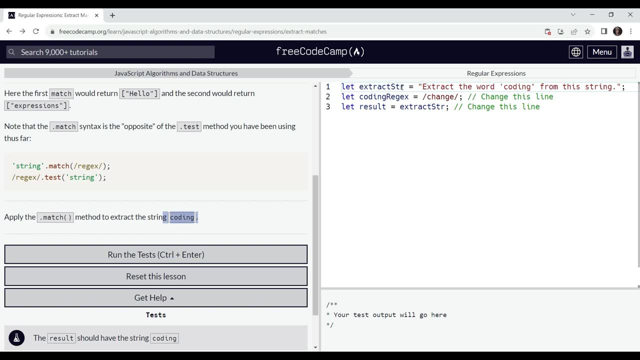 itself. so we're going to look at this example here. it wants us to use the dot match method to extract the coding string from extract str here. so we're going to do that by first changing the change field. here we're going to change that to the coding string as specified in the prompt. 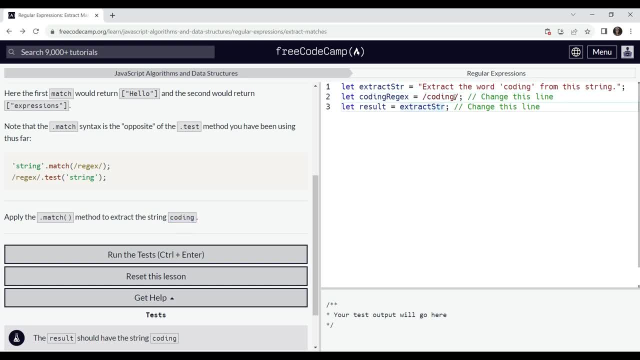 and then next we're going to let the result be equal to the extract str dot, which is the name of the string. dot match within the single slash notation. within that we're going to actually write the same coding string. we're going to run that so that works. and the reason why it works is because 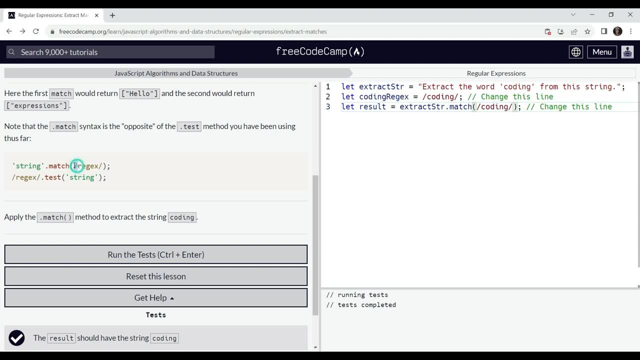 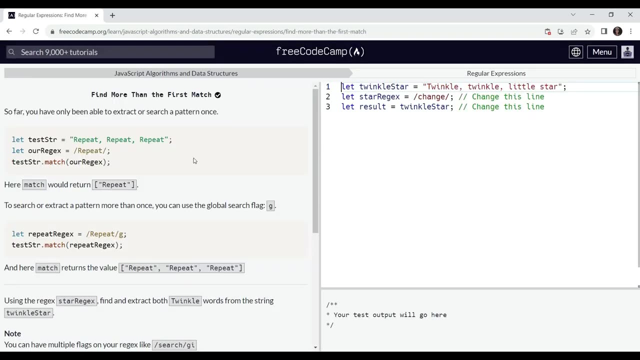 the dot match method utilizes again the single forward slash syntax, as compared to the dot test message, which uses the single or double quotation test method to extract the coding string from the string that was already in the default function, so that we have the function that the key function had. 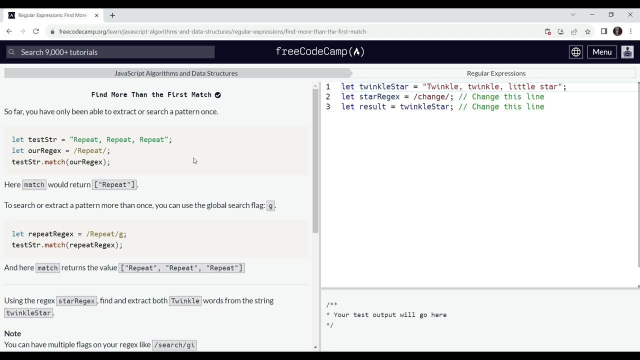 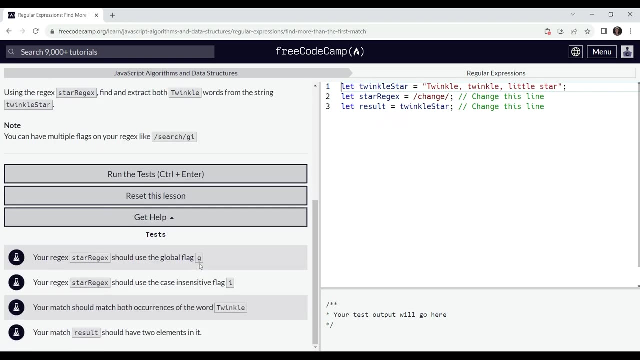 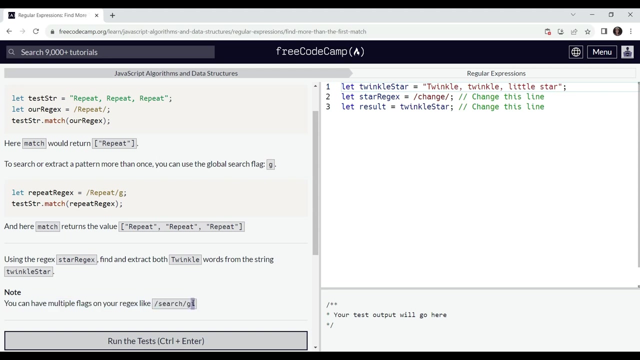 in the format that was already on the object. so we're going to go ahead and do that in the same vein with the dot match function. we're actually going to use now this function to add a flag and the gi flag, remember i being case insensitivity. 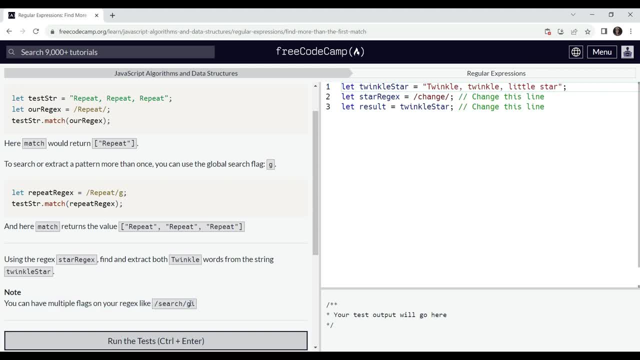 And then G being a global, a global flag. The global search flag allows for multiple extraction of a string. So here with the star regex object, we're actually going to find and extract every twinkle word from the twinkle star String object. 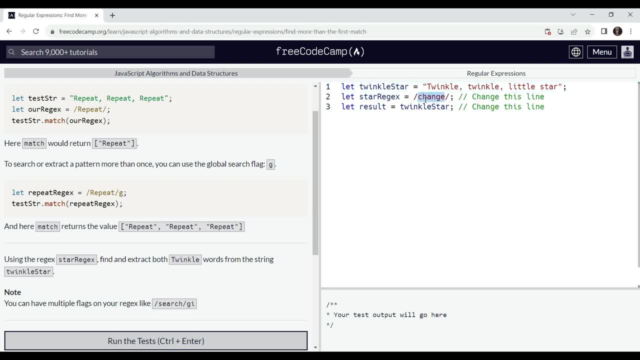 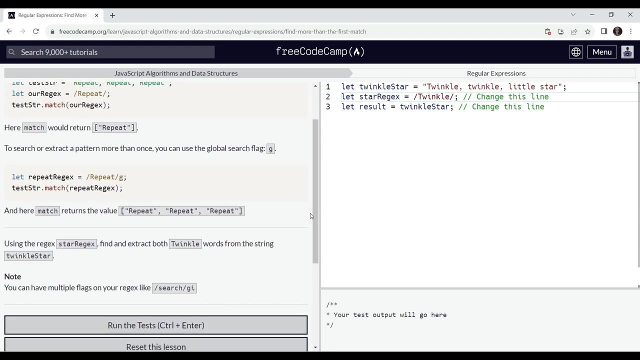 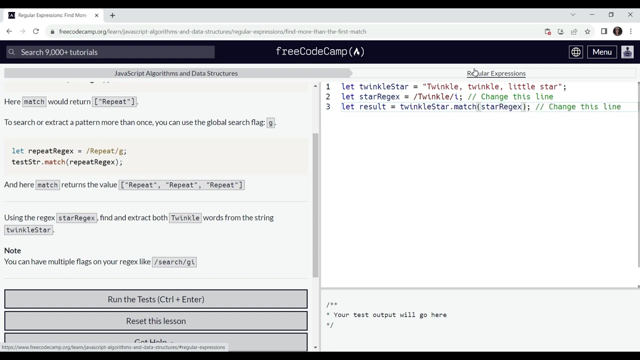 So here we're going to change this to twinkle, Then we're going to add the global tag to it, And then we're going to let the twinkle star string dot match, contained within it, the star regex search string. And before we test this method, we're actually going to add the G global flag as well. as I for ignoring it. 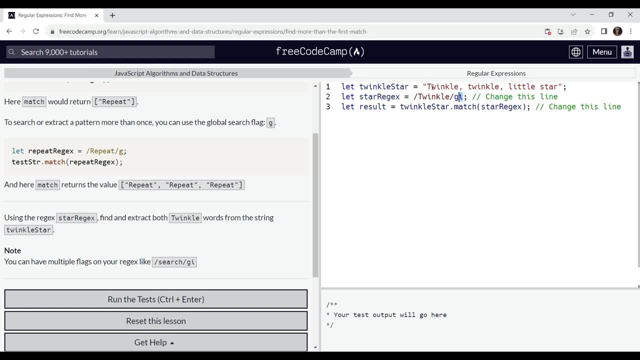 Because we don't care whether we return results with twinkle, with a capital T or a lower key, or whether the twinkle repeats once or is only named once or is contained multiple times in the twinkle star string. We're going to run that and that works. 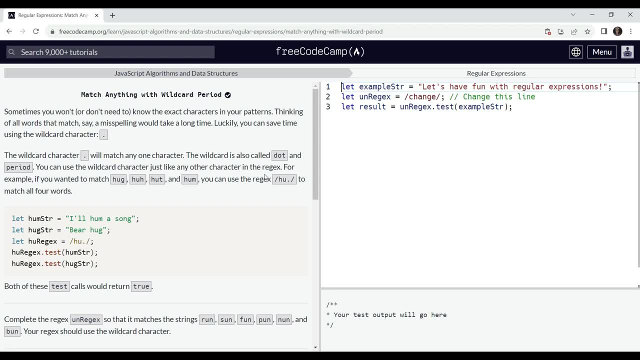 Next we're going to talk about wildcard period notation or syntax. So here we use what's called a wildcard character, which is simply a period in JavaScript to denote any character that doesn't need to be matched within the string in the dot match method. 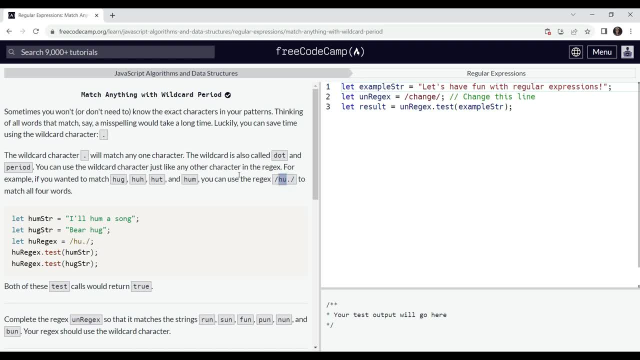 So it specifies here in the example that the first two letters H or characters h and u must be matched, but anything after that, it doesn't matter what the string contains, as long as the string starts with the first two characters h and u, that's, those strings will be returned. 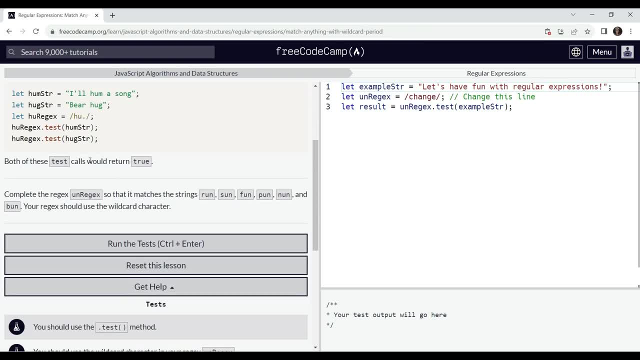 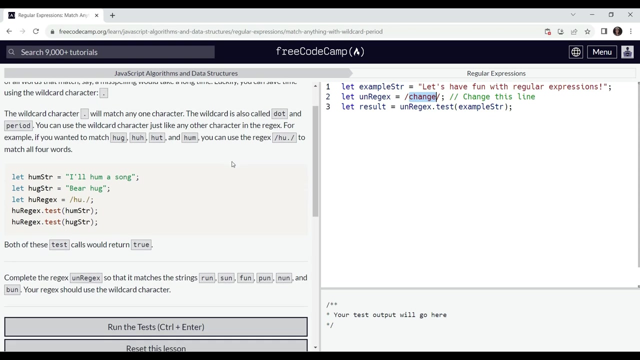 as shown in this example. so here, if we notice the similarity in characters between sun run, fun pun and none, we notice they all end in un. so in this change line we're actually going to include the dot- un syntax, because dot indicates the wildcard character for any. 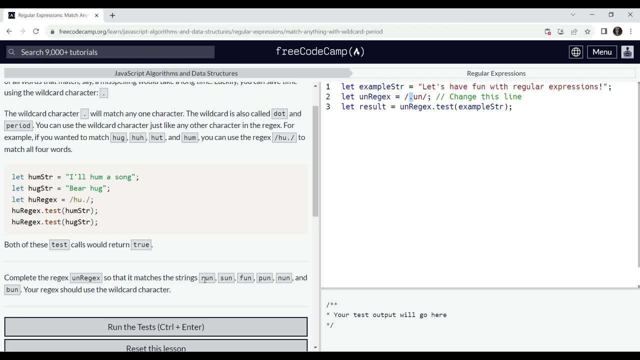 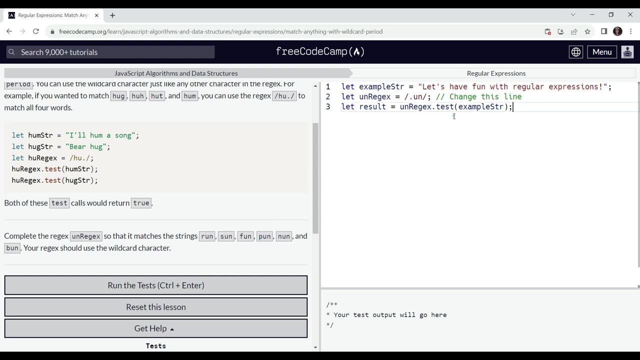 character that any of these strings begin with, such as R, S or F and the UN, is what all the strings end it with And since they're all lowercase and there are no repeating characters, there's no need for the G, the global or the ignore case flags. 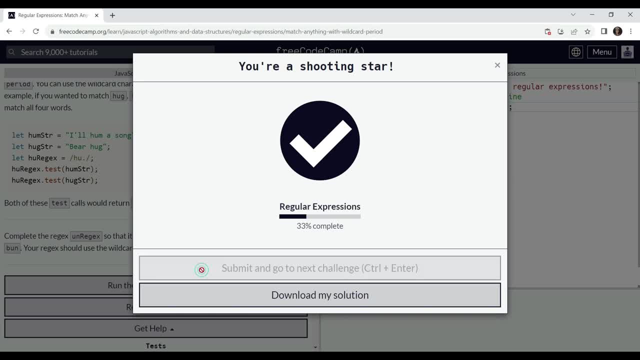 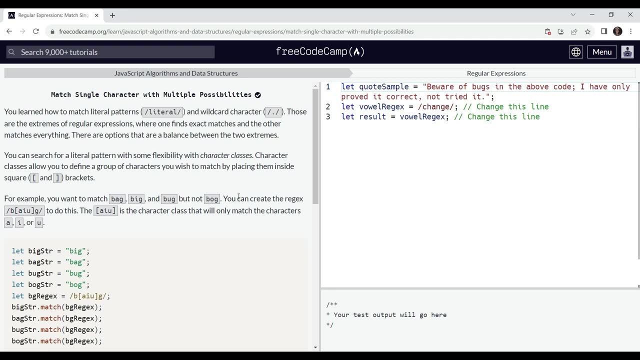 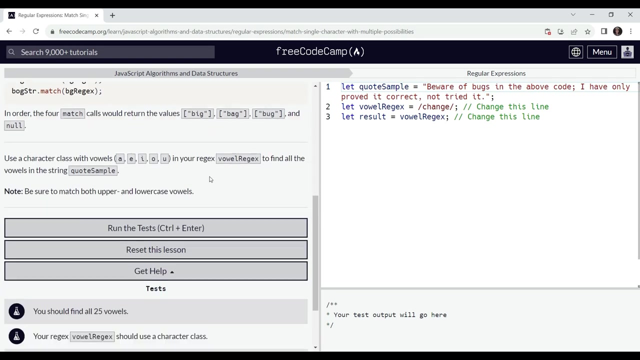 So we're going to run that and it works. So now we're going to use the dot match function to actually match single character, single characters available from a string with different possibilities. Essentially, we want to find the character class with the vowels A, E, I, O and U. 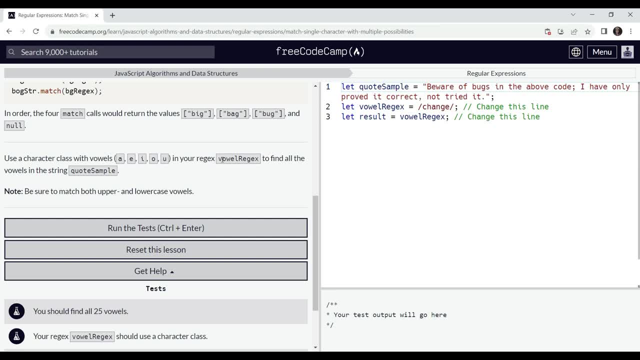 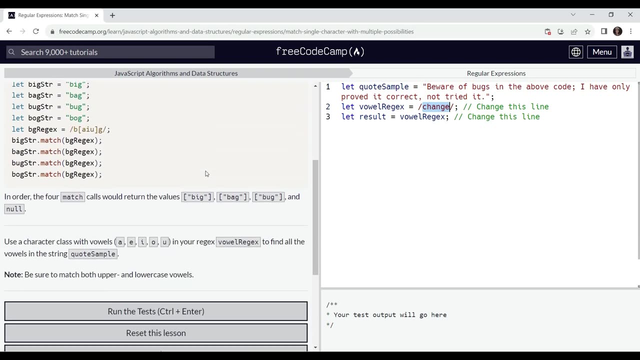 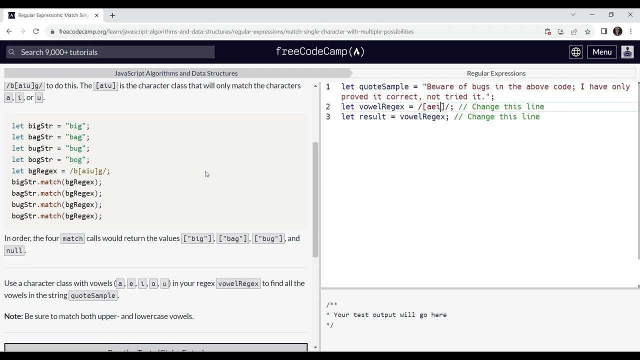 in the regex. So we're going to use object vowel regex in order to find all the vowels contained in the string quote sample. So, following the syntax of the single characters of the vowels, we're actually going to put in here in bracket notation A, E, I, O and U, and then we're going to add the outside. 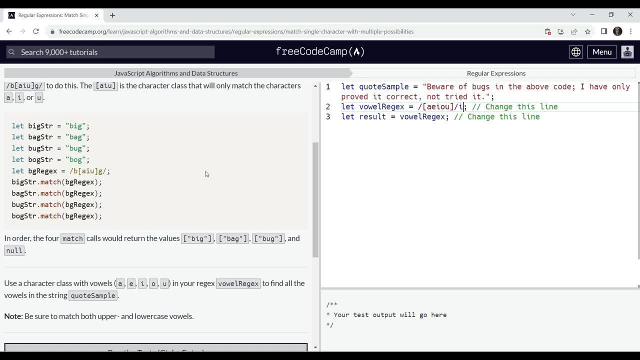 of the single slash, We're going to add I, The I is case- insensitivity flag, because we don't care whether the vowels are uppercase or lowercase in our results. and then we're also going to add the G global flag, because vowels can appear multiple times in the string, of course, and we want to include all of them. 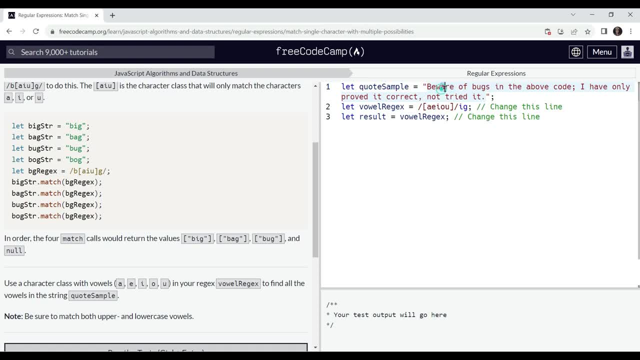 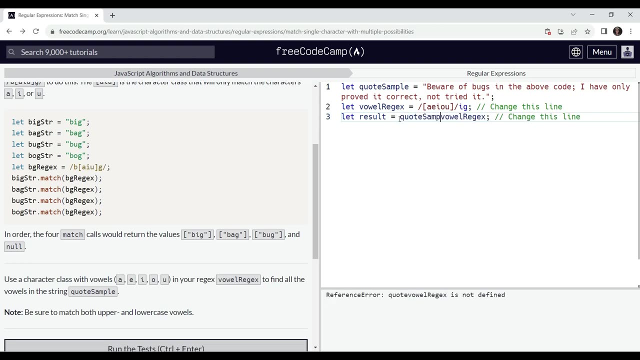 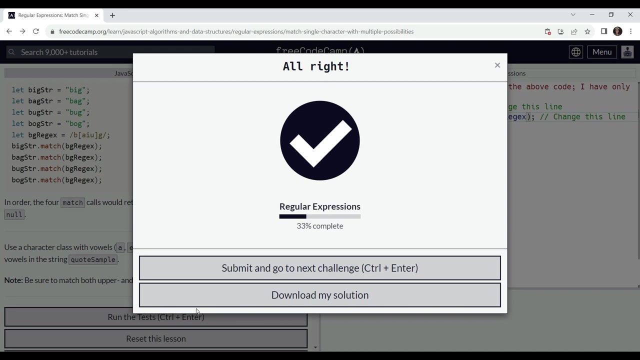 For example, multiple E's here and multiple A's. Next, we're going to actually let the result be equal to quote sample dot match contained within it, vowel regex extraction object. and then we're going to run that and it works. Next, we are going to match letters of the string. 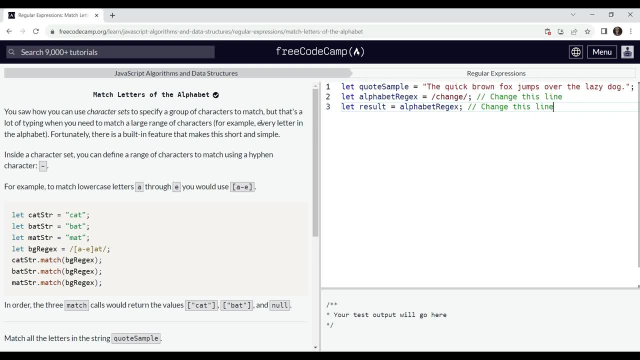 So we're going to do that. Next, we are going to match letters of the string. Next, we are going to match letters of the string. So we're going to do that. So we're going to do that. We're going to add the I to the alphabet with a range syntax using the match function. 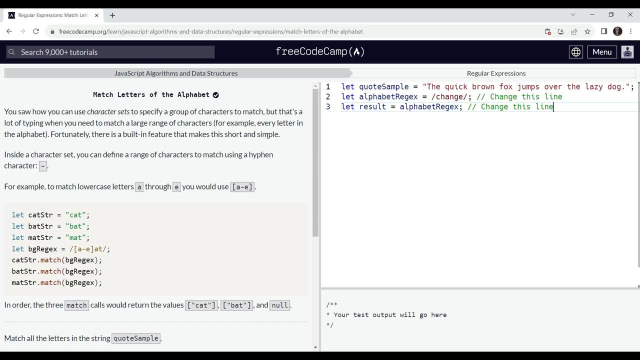 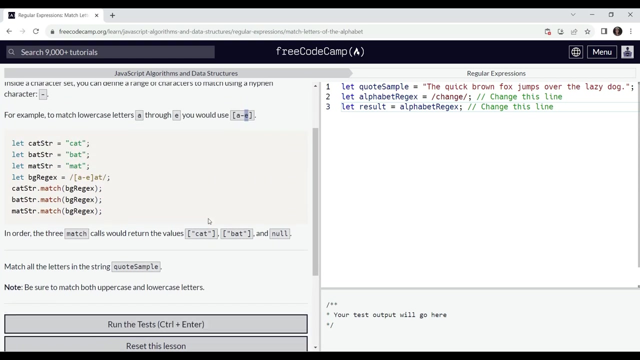 So here we can actually extract individual letters of a string using the hyphen character in bracket notation containing the string with the hyphen- Basically an extraction of a range of strings between A and E in this example. So here they want us to match all of the letters in the string. quote sample here: 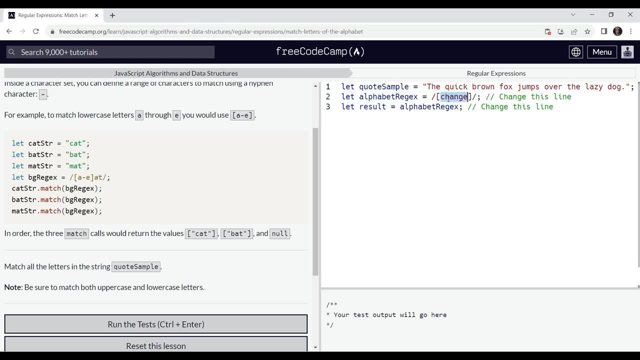 So in the change field we're going to put in brackets- bracket notation- the letters A through Z, because we want every single letter in the alphabet And our result is going to be equal to the string quote sample dot match. 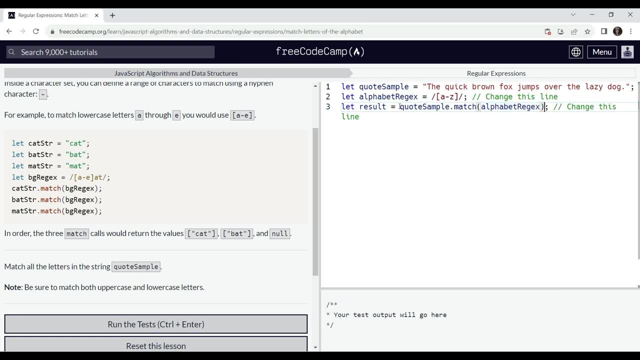 and the alphabet, reg X, search object or string We want to add. make sure that we add the global flag and the ignore case flag at the end, because we don't care about multiple instances of letters and we don't care whether the letter is uppercase or lowercase. 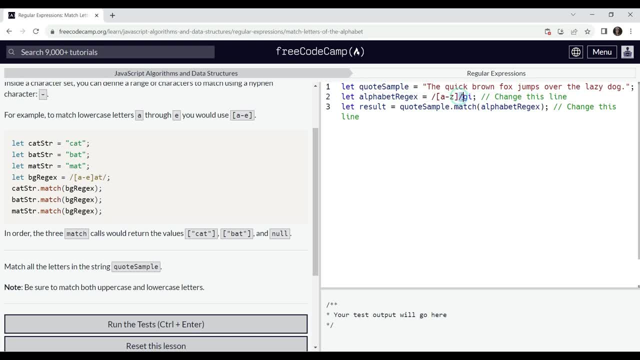 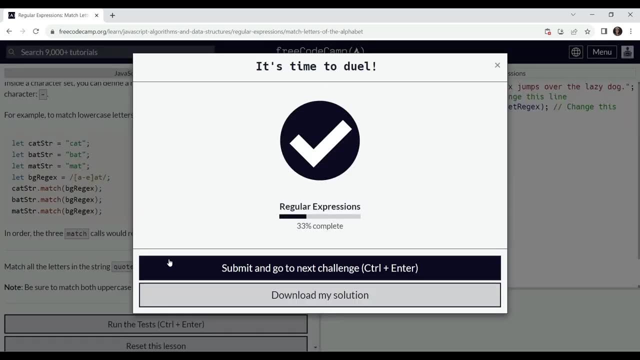 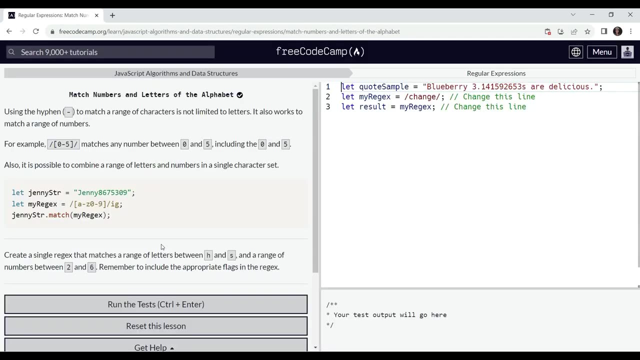 So we want to make sure that we add the GI flags at the end after the forward slash of the string alphabet, reg X. That works. Next we can actually perform a very similar match function with matching both two types of characters, numbers and letters, simultaneously. 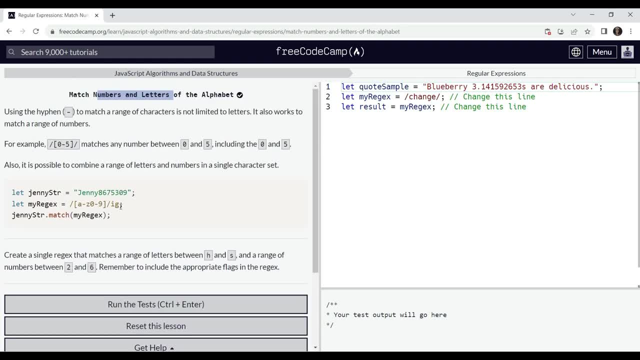 So all we have to do here is basically create a single records, that reg X function that matches a range of letters between H and S. So in this change field we're going to add that here in brackets H, hyphen S, And so we have to include both inside the brackets a range of numbers between two and six. 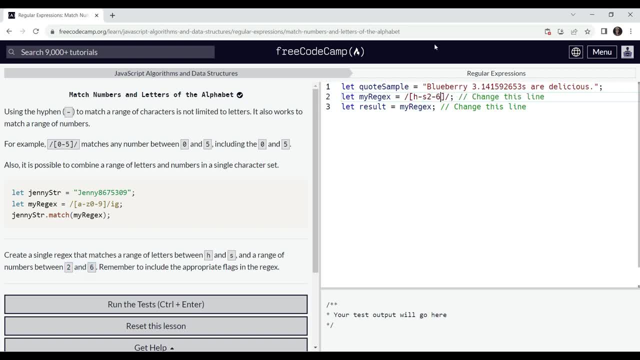 So we're simply going to write that here two hyphen six, And after these single four six, we're going to add that here two hyphen six. And after these single four six, we're going to add that here two hyphen six. 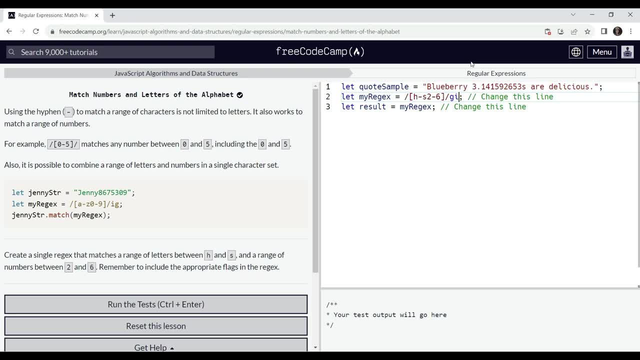 So in this change field, we have to add that here two hyphen six, And after these single four six, we're going to add that here two hyphen six. We want to add the G and the I flags because again, G, global flag. 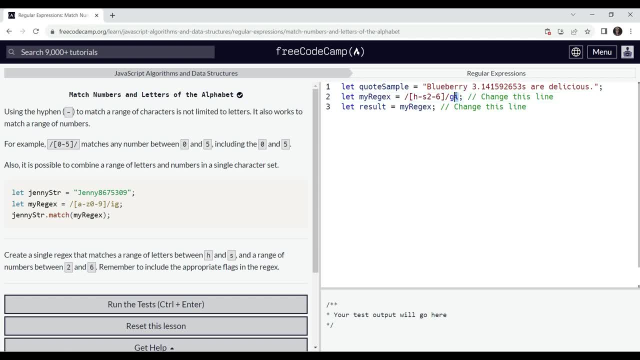 It doesn't matter how many times the characters appear- and I ignore the case of the characters or the letters or numbers- And then we're going to let the result be equal to the string quote sample dot. match Within it the my reg X. 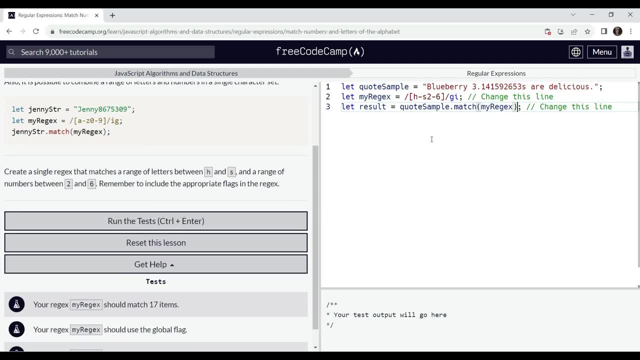 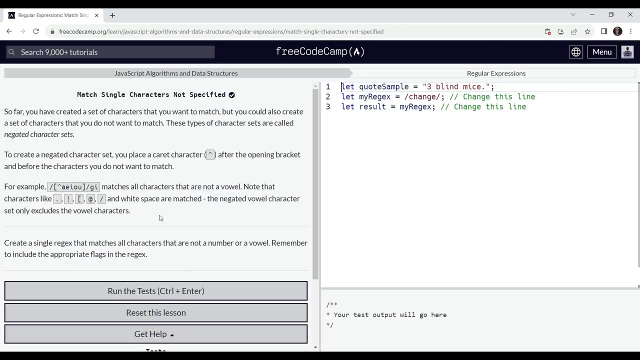 extraction object or string, Which are the ranges of letters and numbers given in the prompt. So we're going to run that and it works. To conclude this tutorial, we're going to talk about the match function for matching single letters that are actually not specified in a string, and